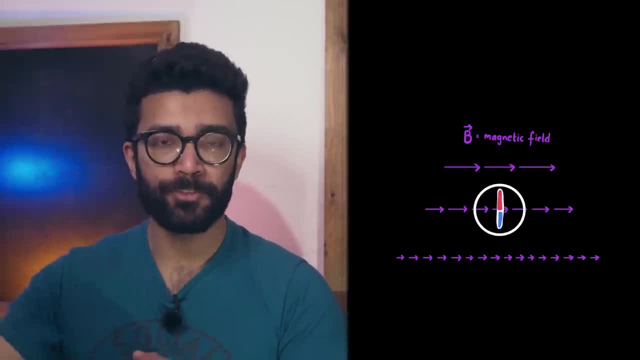 Specifically, the magnet placed in this field will experience forces on it such that its north pole ends up pointing in the direction of the field at every point in space, while the south pole points in the opposite direction. This is because a magnetic field, by convention, points away from. 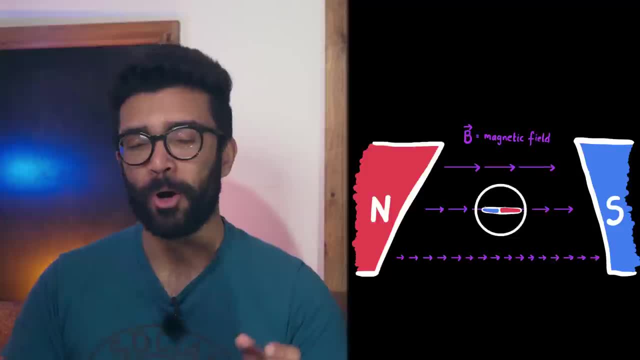 a north pole and towards a south pole And, as we know, opposite poles are the same direction. So the magnetic field therefore shows us what direction an external magnet will end up pointing in, And the magnitude or size of the field also tells us how strong the forces acting on the 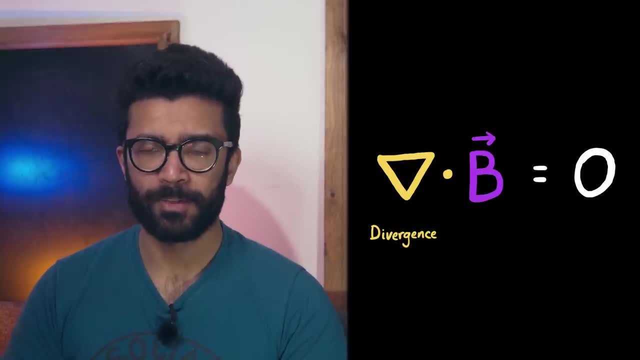 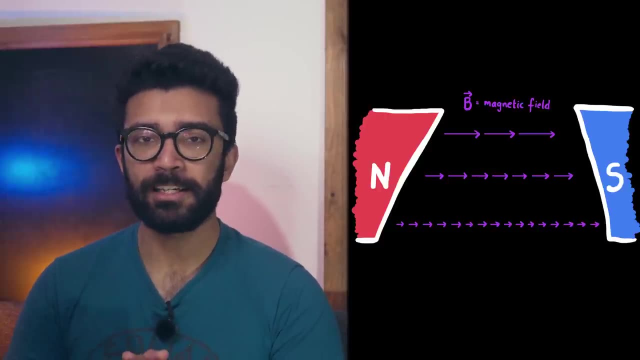 external magnet will be. Now this divergence term is used to measure the net flow of magnetic field through any closed region of space. Basically, if we take any volume we like, let's say this cube- and consider the amount of field pointing in, 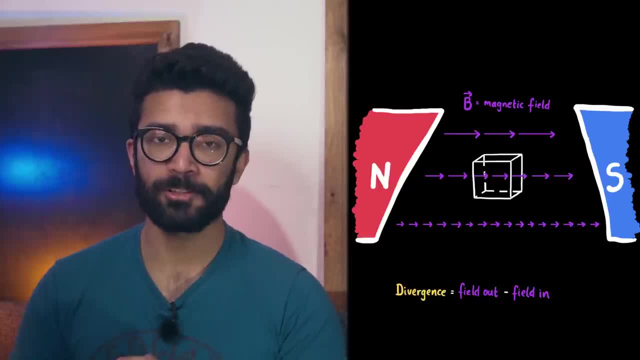 then this exactly balances the amount of field pointing outwards, which is why the divergence is zero. Now, Maxwell's equation says that this is always true for any magnetic field that is allowed to exist in our universe, as well as for any volume that is closed, meaning we consider all. 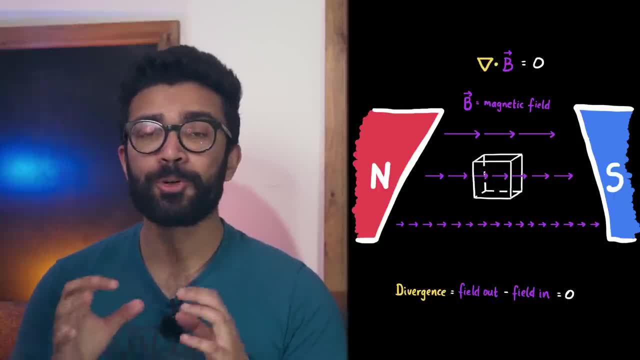 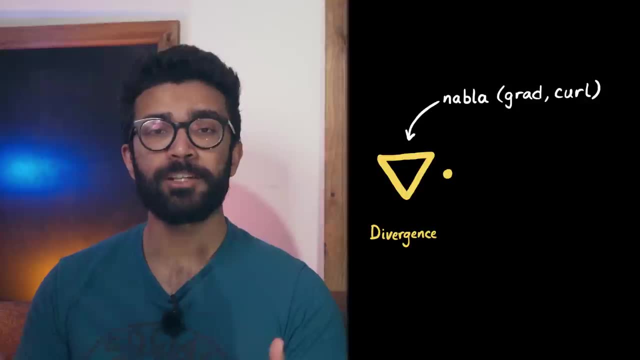 the surfaces around our region of space. For a more detailed description of this, I have a video discussing the downward pointing triangle known as the nabla operator, which can be used to represent two other functions known as gradient and curl, as well as divergence. 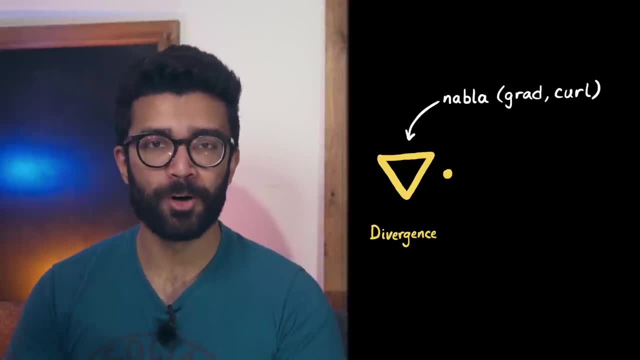 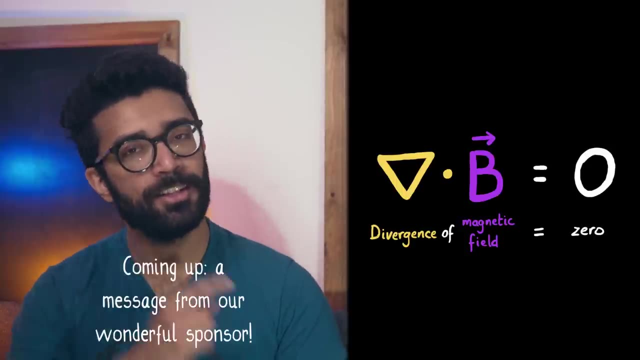 Check out that video up here if you're interested And if you want to know more about this particular Maxwell equation, with visual examples and a more detailed description, then please check out this video up here Now. before we go any further, I want to take a moment to thank the sponsor of this. 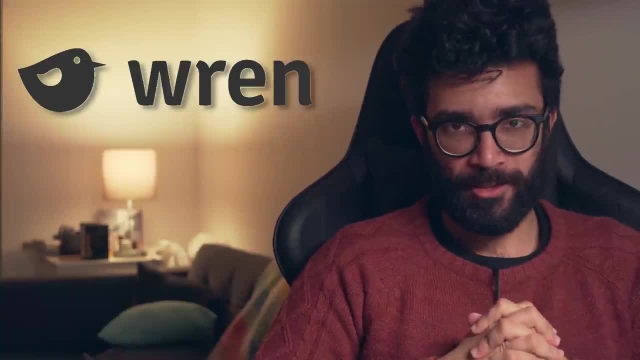 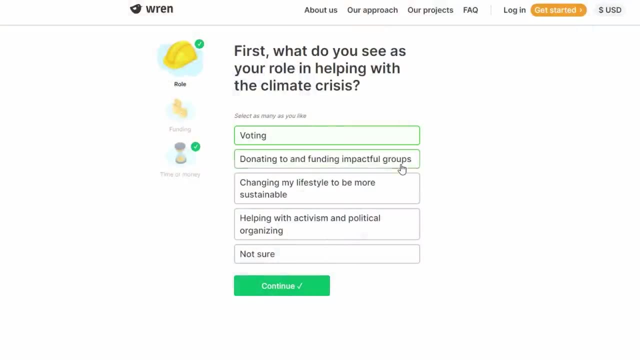 video Wren. We've all heard about the climate crisis at this point, and I think there's something that we can all do to help, whether that's encouraging companies and governments to take it ever more seriously or reducing our own carbon footprint, For example. I've been 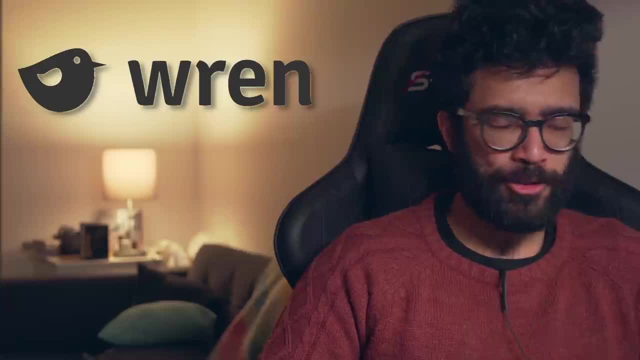 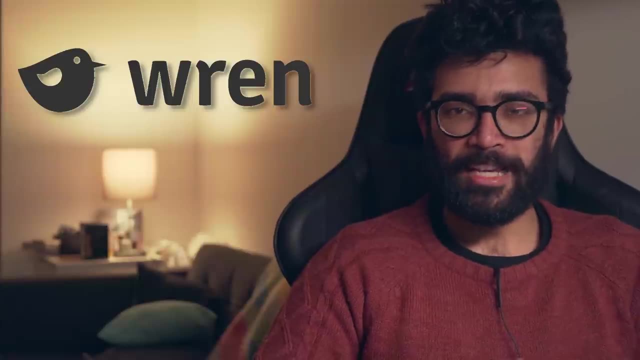 taking some small steps, changing my daily lifestyle to try and reduce my carbon footprint a little bit: walking more often than driving, cutting down on meat consumption, making responsible purchases and so on. So I was very happy when Wren got in touch with me asking to sponsor one. 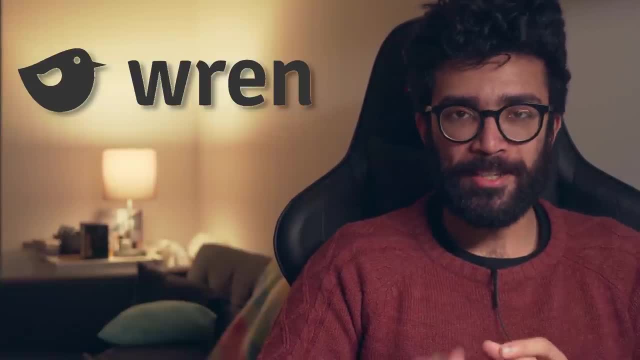 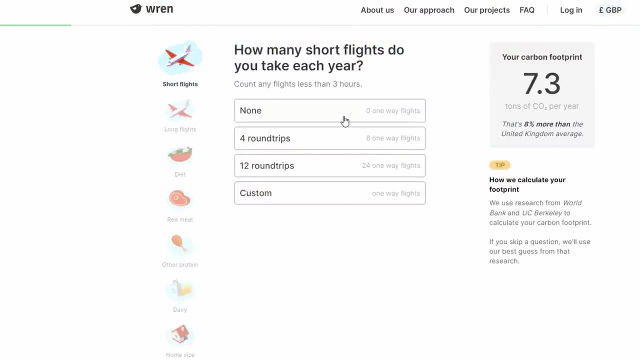 of my videos. Wren is a simple but effective way to make a difference in the climate crisis. Their website, linked down below, allows you to calculate your own carbon footprint and then gives you ways to reduce it. You can also make a monthly contribution to offset your 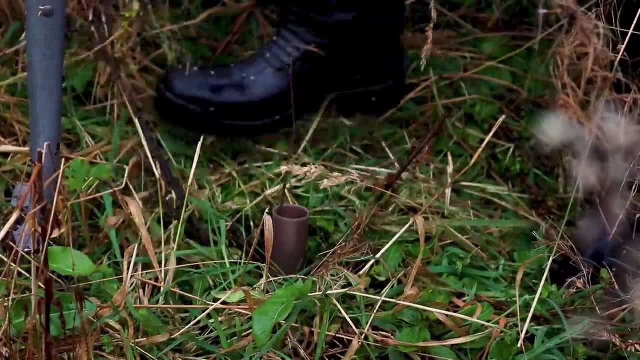 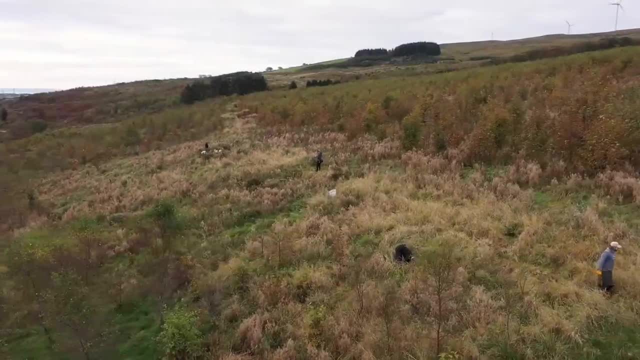 footprint by funding diverse carbon reduction projects like tree planting, mineral weathering and rainforest protection, And Wren will then meticulously quantify what impact each project is having and send you monthly updates so you can be sure that it's making a difference, Wren. 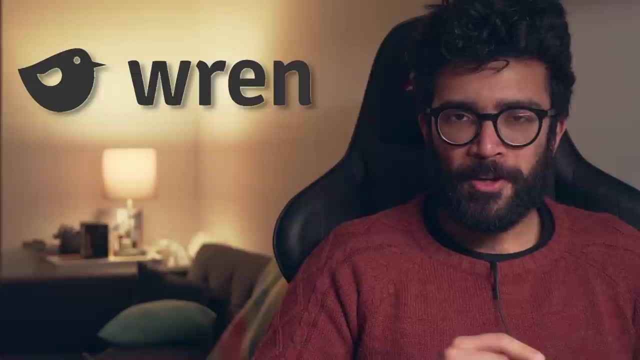 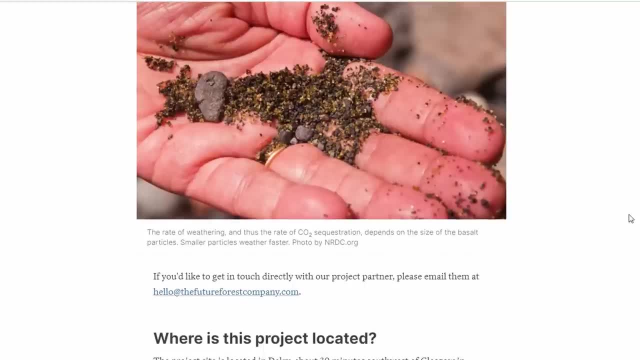 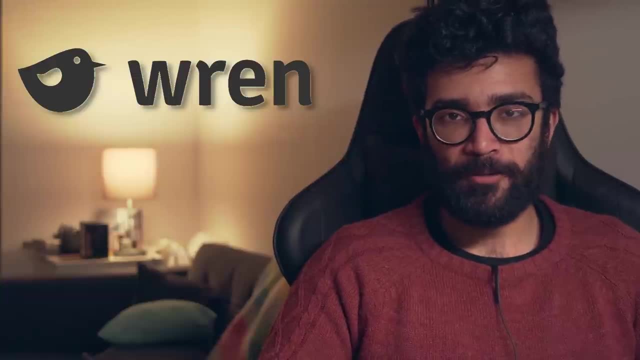 As well as this, these projects need to have not just a positive impact, but a measurable one, so that we know exactly how much CO2 is being offset and that it will stay out of our atmosphere for a long time. On top of this, Wren is a benefit corporation with a legally binding charter. 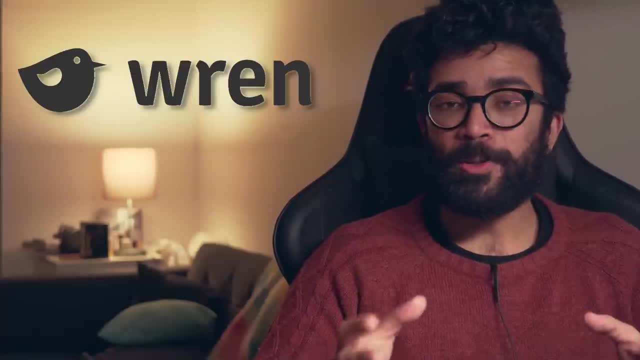 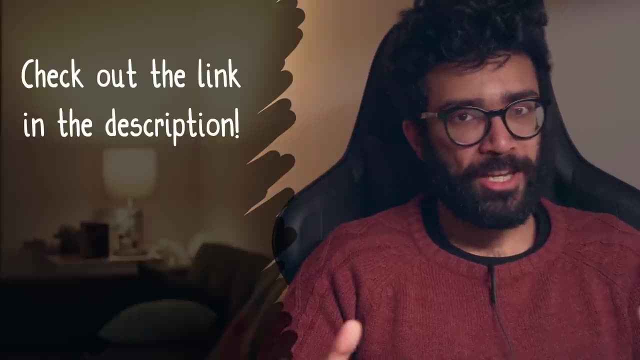 meaning their work is as transparent as possible. So if you'd like to calculate your carbon footprint and find out a bit more about Wren, then click the first link in the description box below. It helps the channel out, of course. and the first link in the description box below: 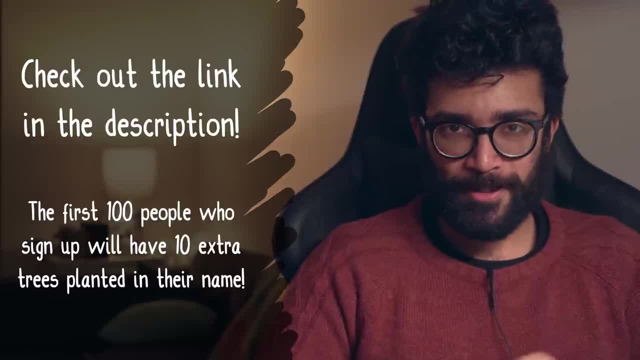 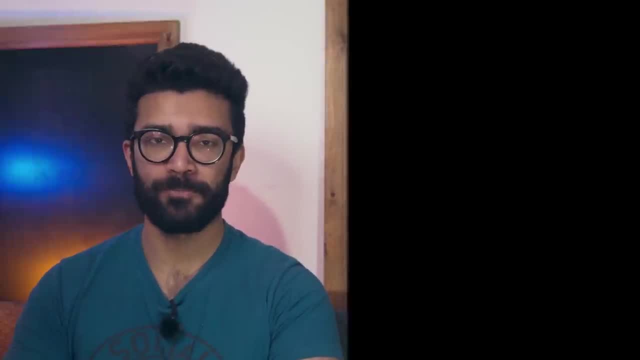 The first 100 of you to sign up will get 10 free trees planted in your name. Huge thanks to Wren once again for sponsoring this video. Let's move on to looking at another equation and the mathematical language used within it. The second one of our Maxwell equations looks like this: Once again we see our friend, the 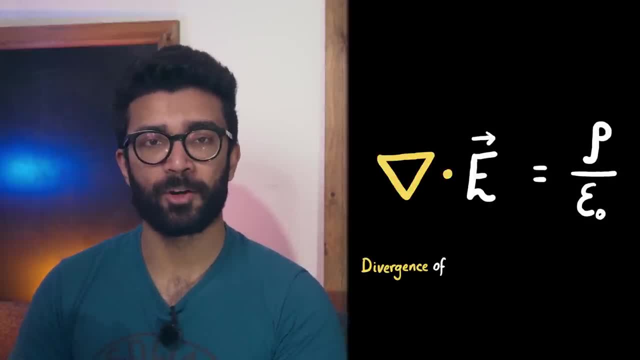 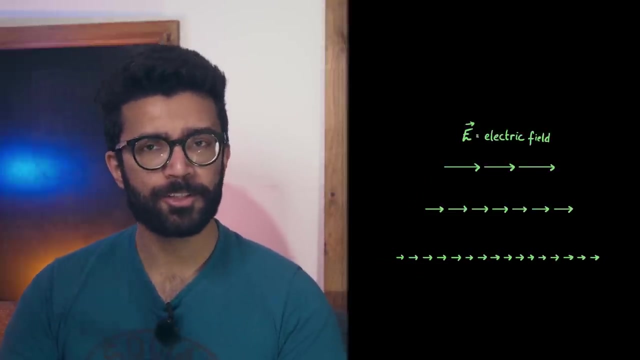 divergence operator, but this time we're taking the divergence of the electric field E, And we can see that this quantity is not equal to zero. Let's look at what the right hand side of the equation says in a moment, But first let's take a quick look at the electric field. Similar to a magnetic field, the electric 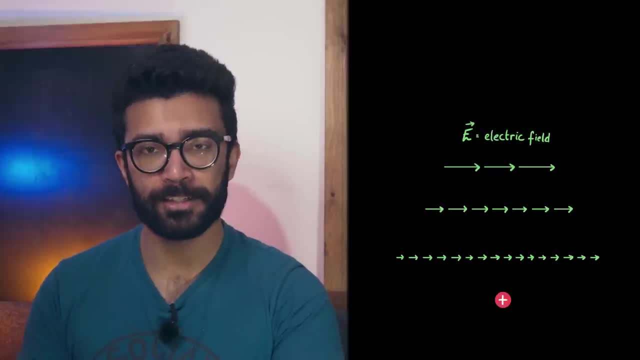 field shows what happens to electrically charged objects placed within the field. If we take a positive charge and place it here, for example, then it will experience a force in the direction of the field lines And the strength of that force depends on the strength of the field given by the 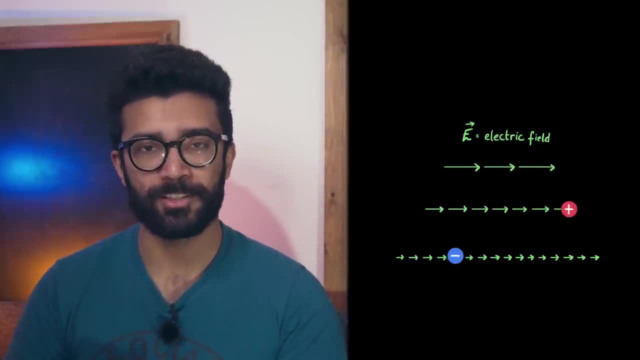 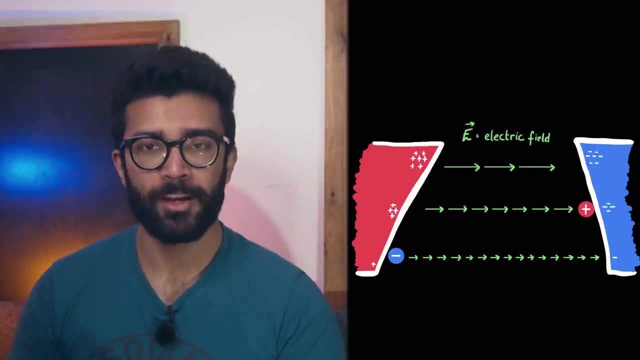 size of these arrows And a negatively charged field will have a force that is equal to zero And a negatively charged particle will experience forces in the opposite direction. An electric field begins at a positive charge and ends at a negative charge. Therefore, we can see. 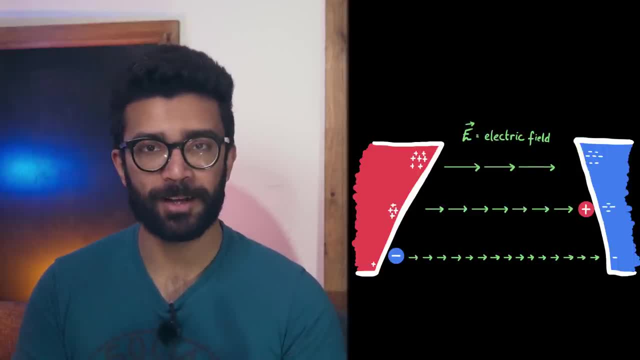 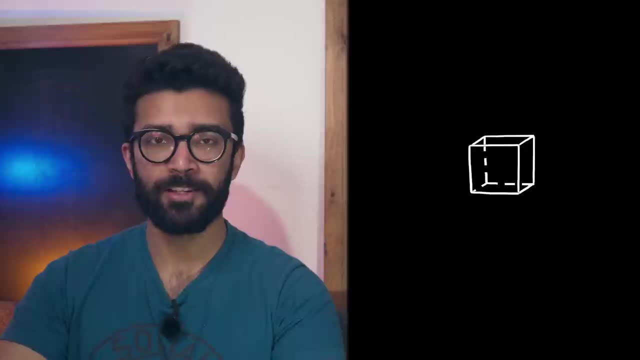 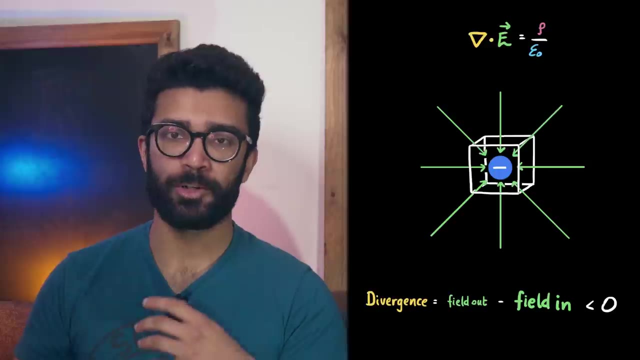 that opposite charges attract. in this model, just as we expect Now, it looks like the divergence of our electric field is non-zero. This means that if we choose a region of space, it is possible for the total amount of electric field pointing into that region to be bigger than the amount pointing out. 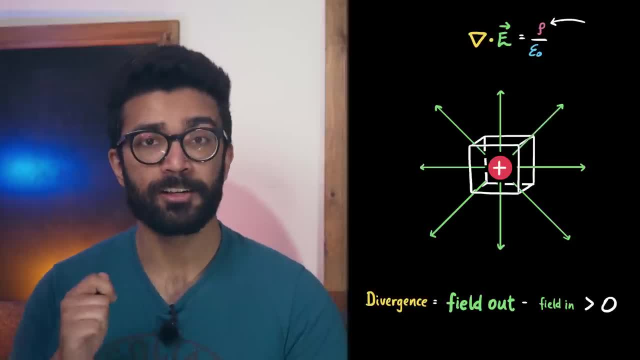 Or vice versa. What it depends on is this: quantity: rho. Rho represents the charge density or the charge per unit volume within the region of space that we're considering. The larger the charge density, the more charge packed into our volume, the larger the divergence. 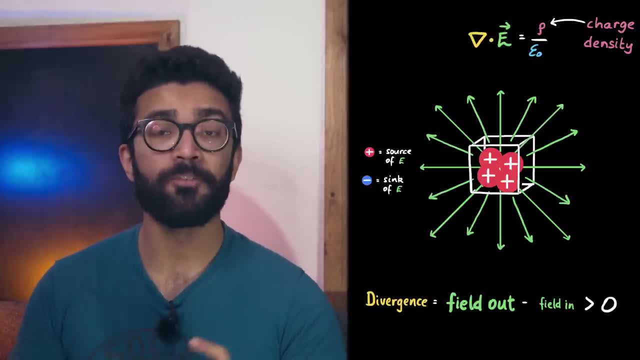 Because charged particles are sources or sinks of electric field, right? So the more of them we have in our region of space, the larger the net effect of the field pointing outwards. The signs simply tell us whether we have more outward pointing fields generated by 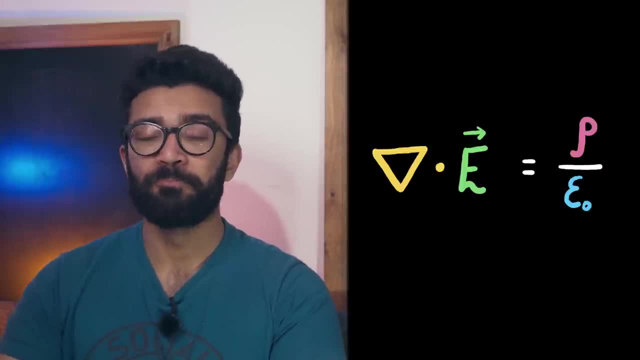 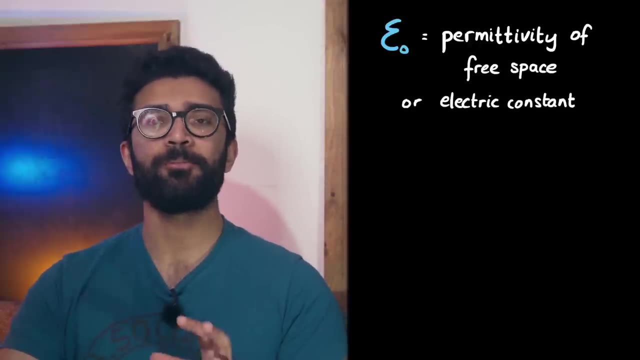 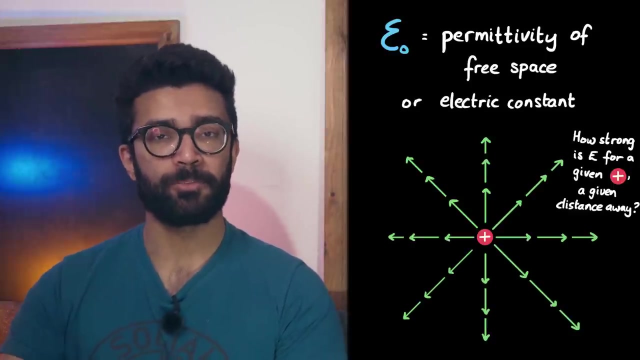 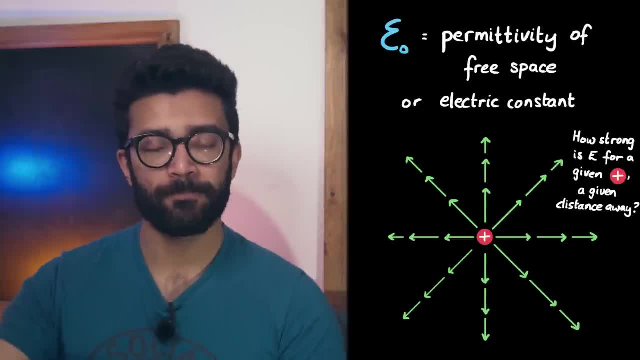 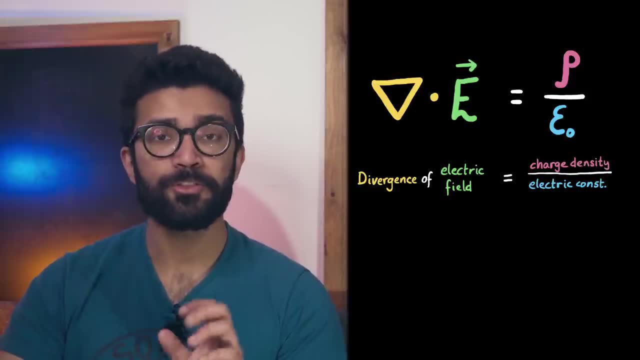 with the size of the electric charge generating it and how far away from the charge we are. So that's the second Maxwell equation briefly discussed. It's interesting that electric fields and magnetic fields behave slightly differently, so check out this video up here for a more detailed. 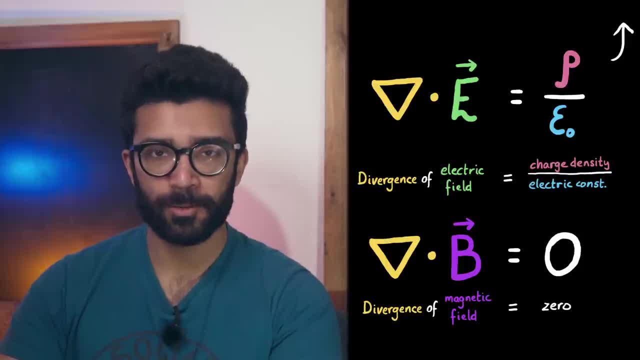 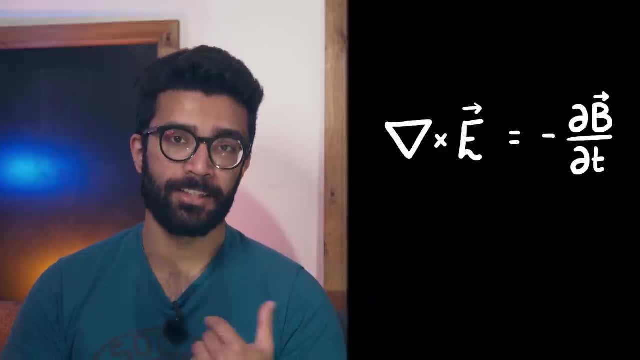 discussion of the second Maxwell equation. Let's move on to the third one, though, and again look at the mathematical language, the terms used in it. The third of these equations looks something like this: We read this as saying that the curl of the electric field is equal to negative, the rate of 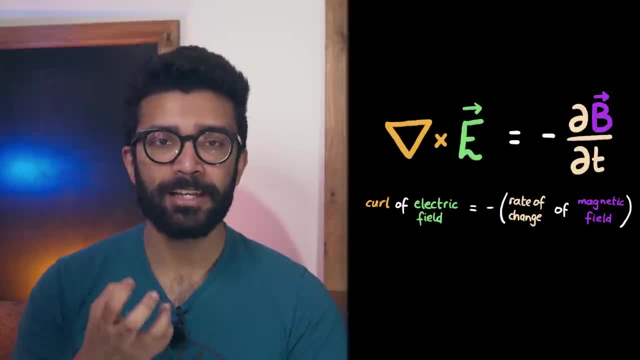 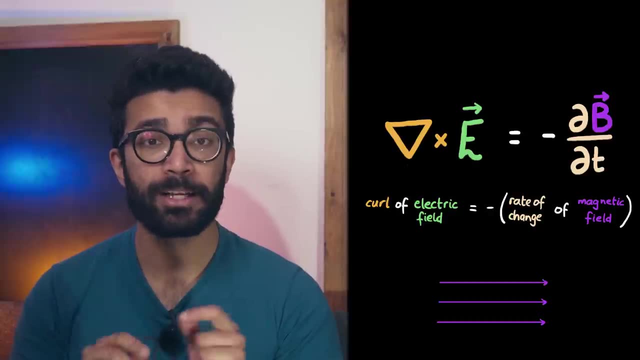 change of the magnetic field. So this equation now links together electric and magnetic fields with each other. The right hand side is a measure of how quickly the magnetic field we are studying changes over time. The faster it changes, the larger the value of db by dt and the negative. 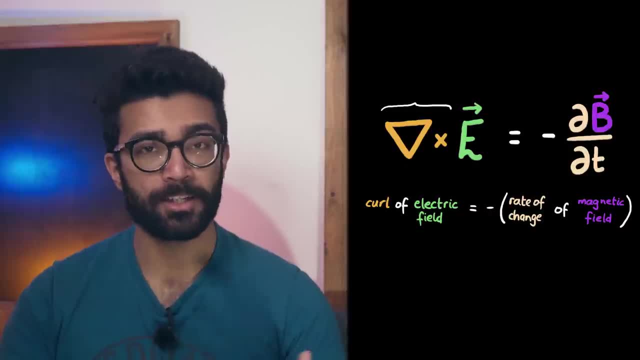 of this rate of change must be equal to this operator curl applied to the electric field in our system if the system is to be something we can find in our universe, Assuming Maxwell's equations do actually describe our universe accurately. Now this operator curl looks a bit like the divergence operator from earlier. 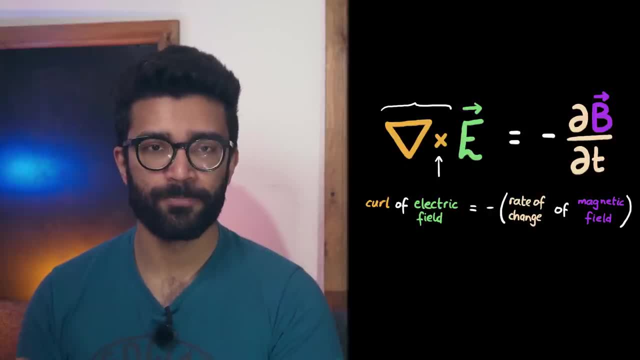 but this time we have a cross here rather than a dot. There's a reason. both the divergence and the curl operators use this downward pointing triangle, this nabla, as part of their notation. Again, that's fully explained in my video about the nabla operator, but curl actually. 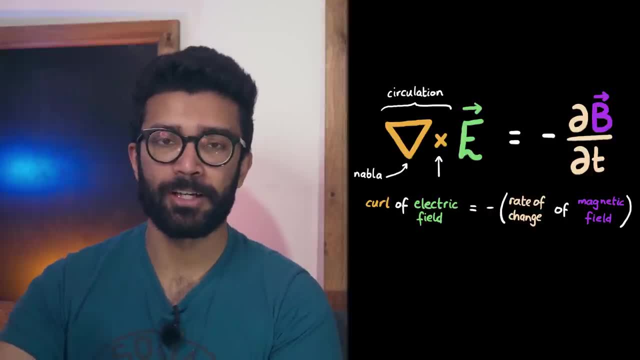 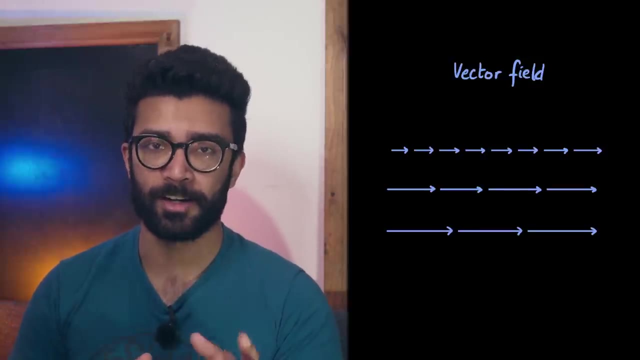 measures what is known as the circulation of our electric field. This is difficult to visualize for electric fields, but much easier to understand if we think of a different vector field, which is something that can be described by a vector at every point in a region of space, so that it has both size and direction. 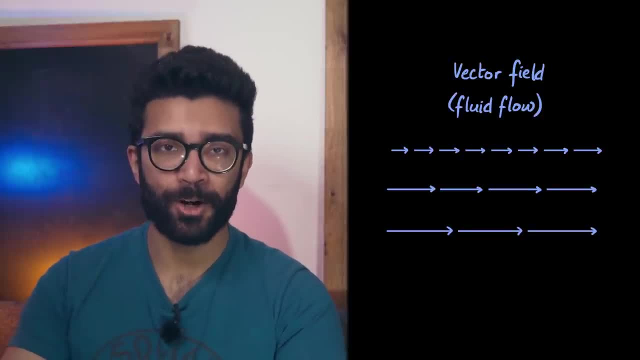 The vector field we'll think about is one that describes the flow speed of a fluid. Large vector means fast flow, small vectors mean slow flow and the direction just gives the direction of the flow. Now, the curl of this vector field can be thought of as what would happen to a little. 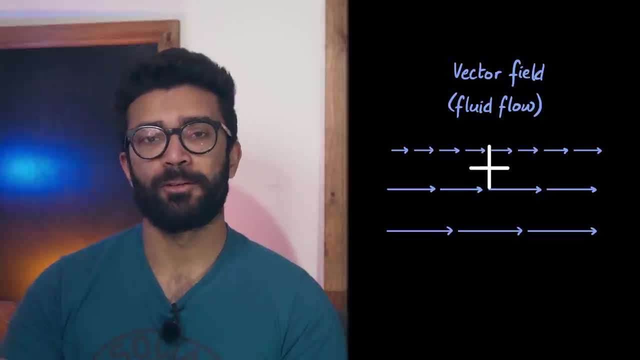 fan that we drop into the fluid At this point, for example, the fan would rotate this way and fairly quickly, because this flow is much faster than this flow. So the curl of the field measures this circulation and its direction. This is much more tricky to understand in a simple physical way for the electric field. 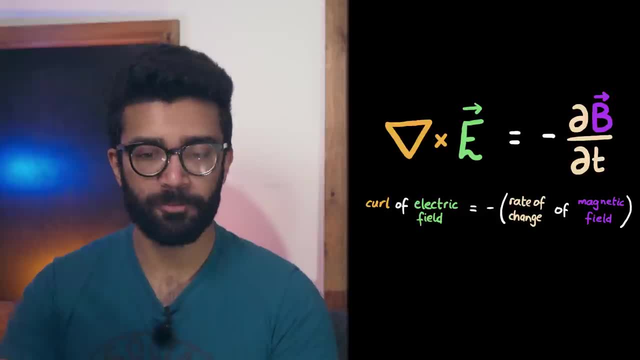 but the curl is a useful indicator of the properties of any electric field we study. How it behaves can be indicated by its curl, and the curl must equal minus dB by dt. Another way to think about this is that an electric field can be generated with these. 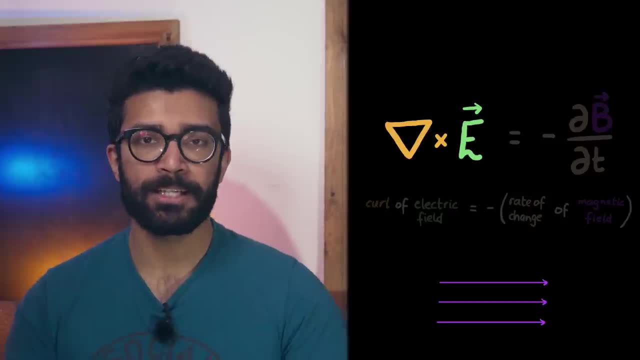 specific properties with this specific curl, If we have a magnetic field that changes over time with this particular rate. Again, for more details, check out my full video on this Maxwell equation. But for now let's take a look at the final one. 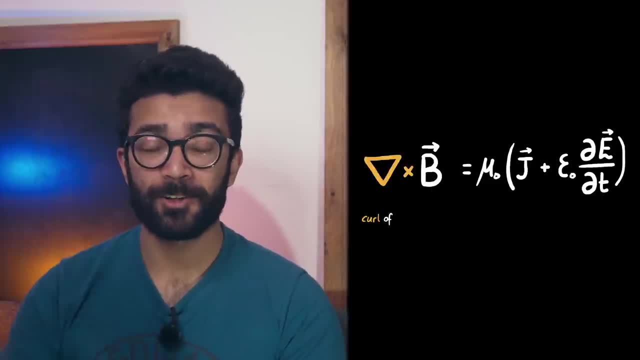 It looks a bit like this. This time we see the curl of the magnetic field and how it relates to the electric field. in the system that we're studying We see this term epsilon-naught from earlier, as well as the rate of change of our electric. 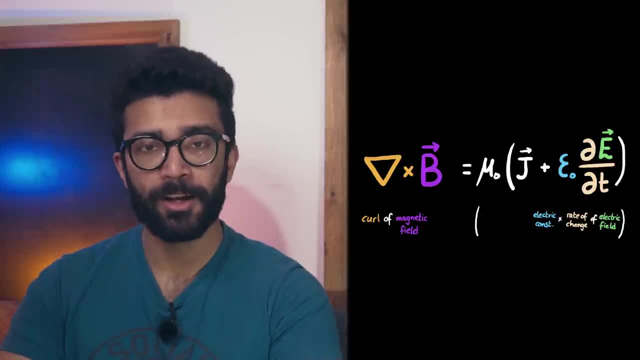 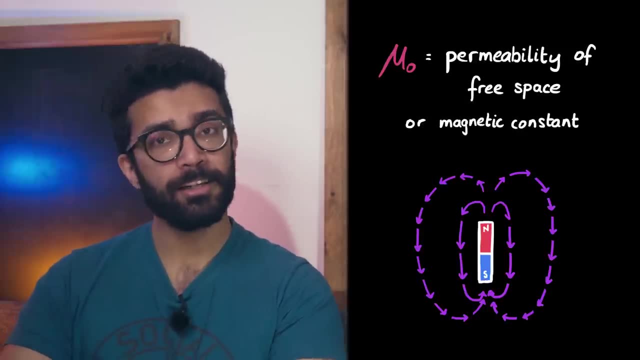 field, or how quickly the electric field changes over time. But now we have two different fields, Two new terms here: mu-naught and J. Mu-naught is known as the permeability of free space or the magnetic constant. So it's basically the magnetic version of epsilon-naught in many ways. 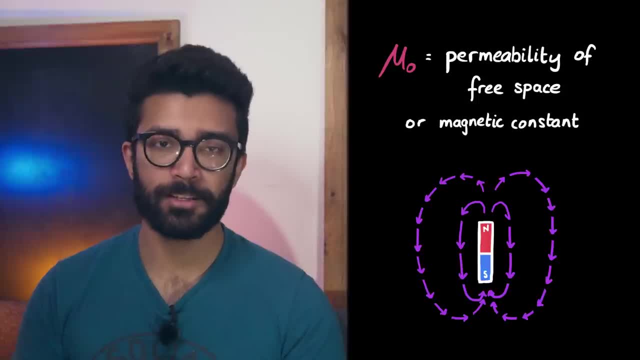 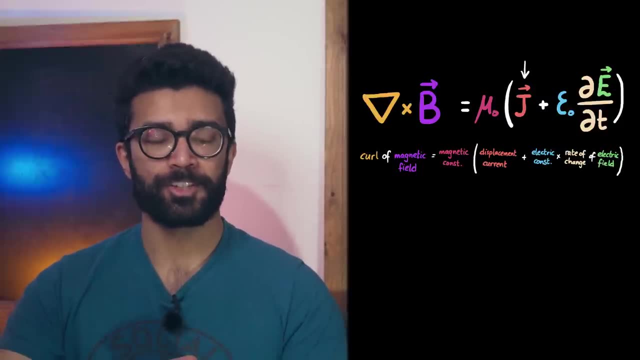 It determines how magnetic fields can exist within empty space for magnets of given strengths. And finally, this quantity J is Maxwell's addition to an equation that already existed but wasn't quite accurate enough. It's known as the displacement current and basically represents the current passing through. 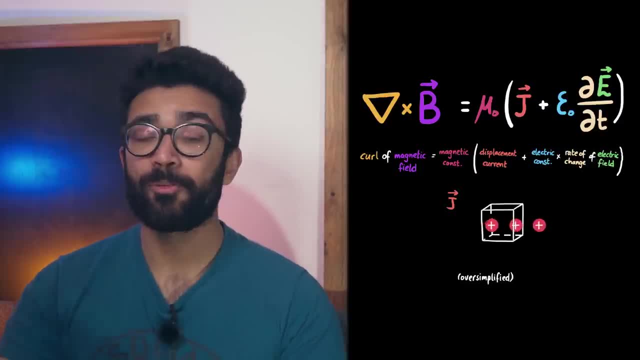 any surface around the region of space we are studying Now. remember, current is just a flow of charged particles. So, in a very simplified manner, without going into too much nuance, this equation says that a magnetic field can be generated by a changing electric field within our region of space. 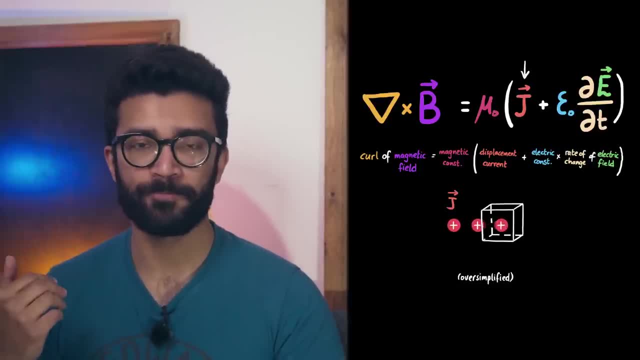 or a flow of charged particles into or out of our region. There is a lot more nuance to this equation, But let's take a look at the next one. So this equation says that a magnetic field can be generated by a changing electric field within our region of space or a flow of charged particles into or out of our region. So this equation says that a magnetic field can be generated by a changing electric field within our region of space or a flow of charged particles into or out of our region. But let's take a look at another equation that I'll cover in a future video. 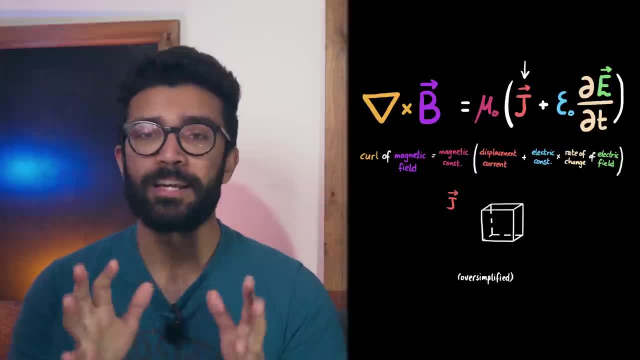 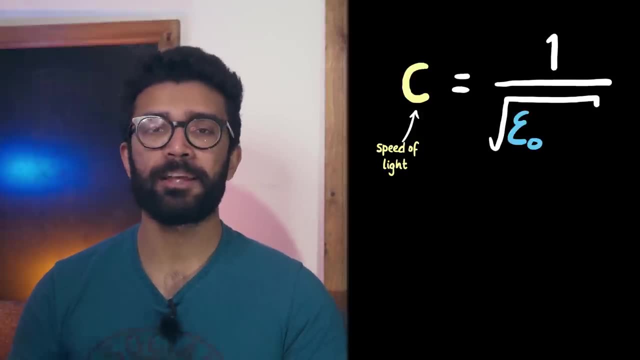 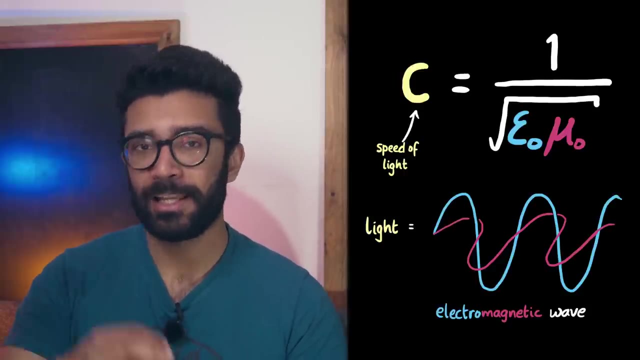 which will be the final one in this Maxwell equation series. Now here's a fun fact before we finish up. The speed of light in vacuum is directly related to the permittivity and the permeability of free space, Because light is an electromagnetic wave, and these constants tell us how electric and magnetic fields should behave in a vacuum. 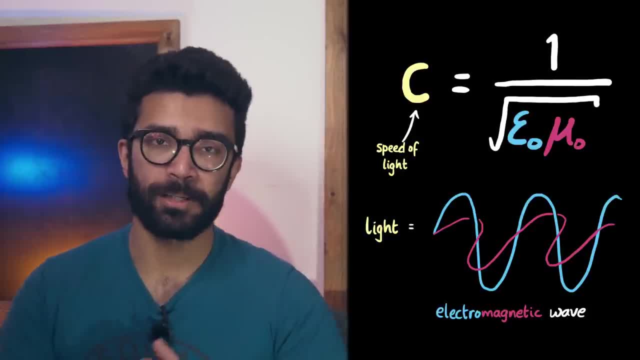 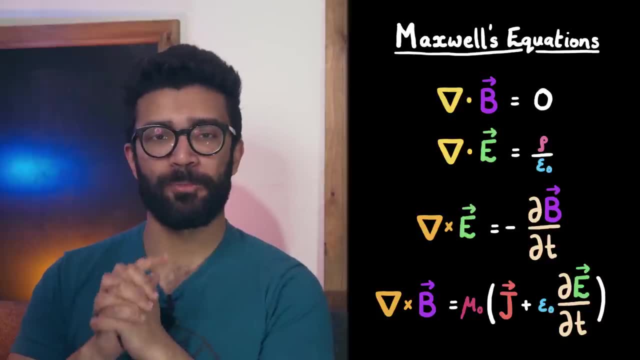 therefore, electromagnetic waves travel at this speed. And with all of that being said, we've briefly touched on all the math we need to know about the frequency of light in the vacuum, on all the mathematical language used in Maxwell's equations of electromagnetism.